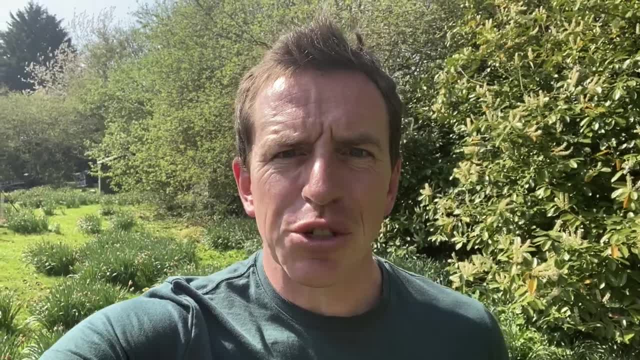 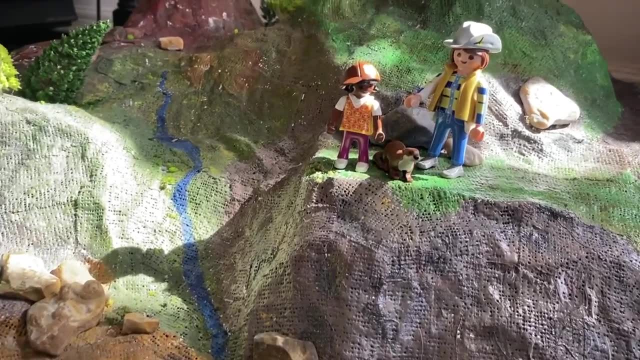 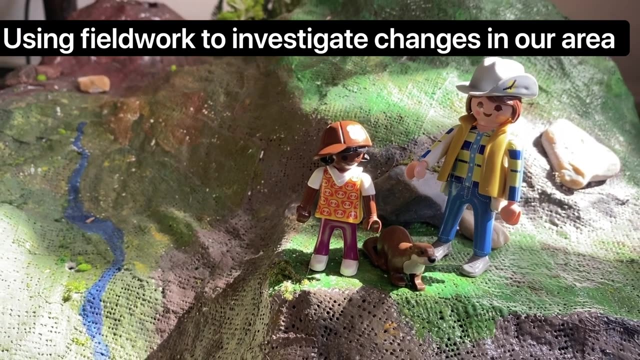 of us over the last few weeks. the world has shrunk In years to come. people might ask you: how did your area change during the coronavirus lockdown? Well, we can use fieldwork to find out. You can use fieldwork to gather real evidence of how your area is changing. 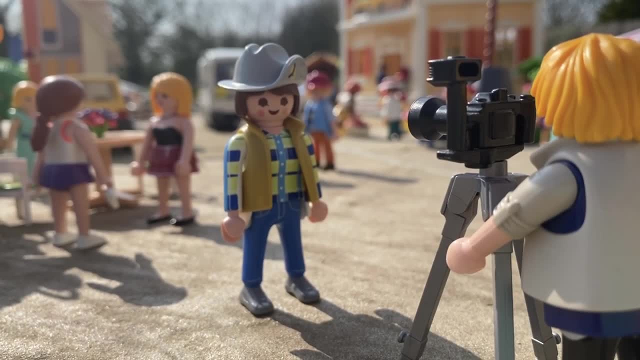 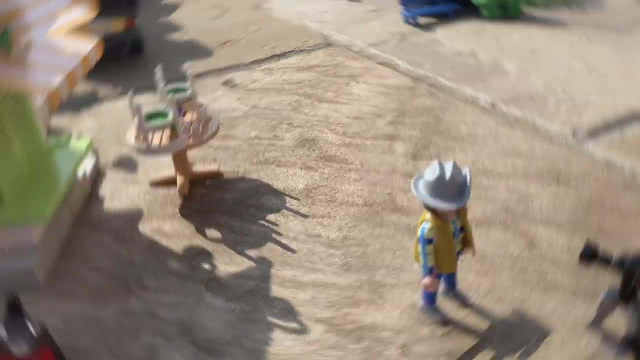 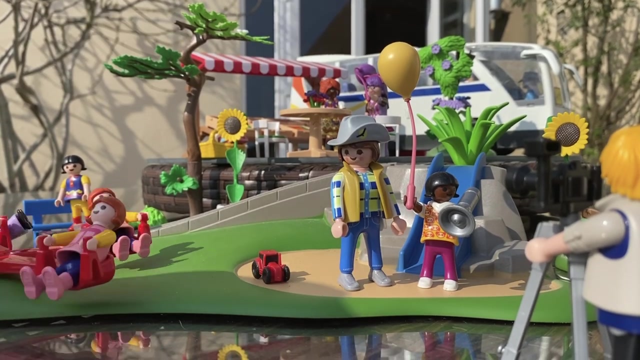 And things are changing. Streets like this one that are usually busy are now deserted. Firstly, we need names. By this we mean what are we aiming to find out, And our aim is: how did the coronavirus lockdown impact my area? 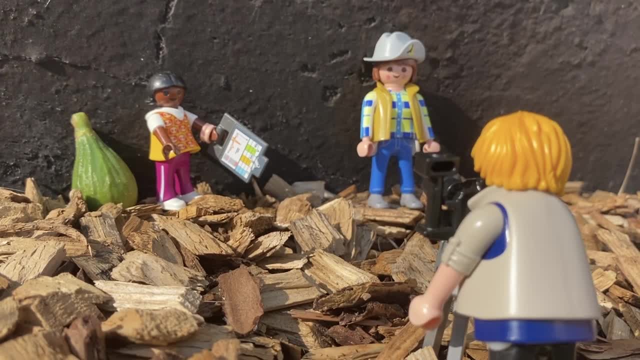 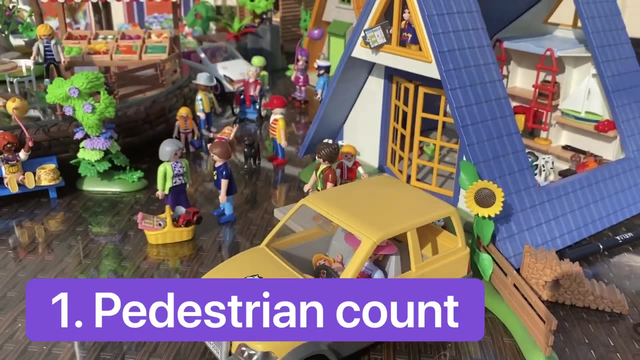 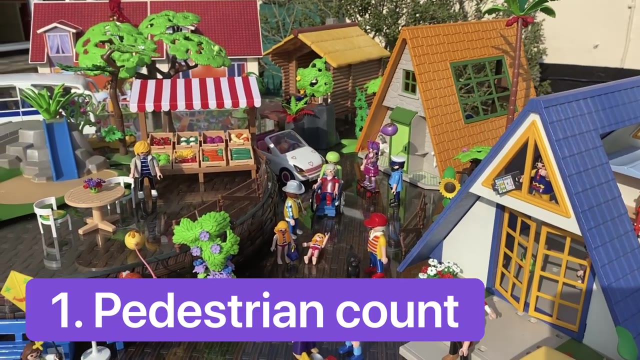 And to find the answer to this. these are some of the fieldwork methods you could try. Number one: a pedestrian count. For this count the number of people you can see from your house over a 60 second period. You might expect this will be less at the moment than normal. 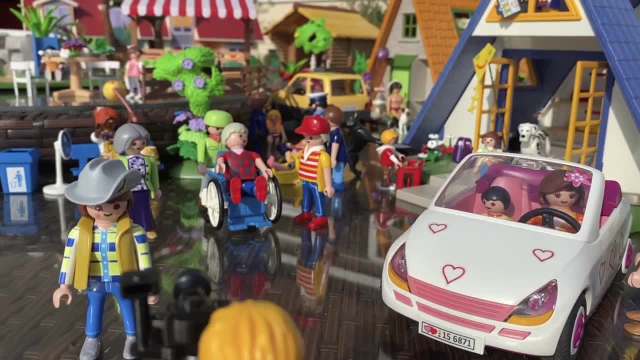 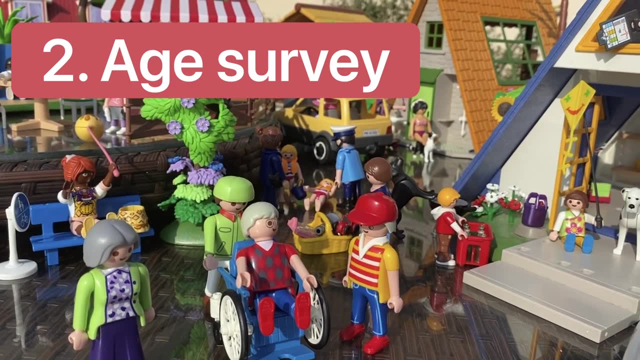 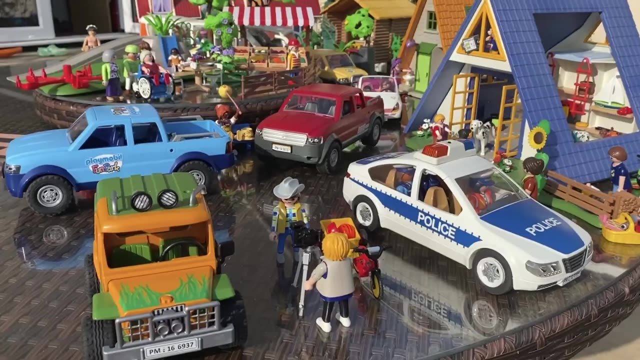 Number two: another thing you can do is an age survey. For this one you could count the number of children, teenagers, adults and the elderly. Again, you might expect there to be less old people about at the moment. Number three: a transport survey, Again over a 60 second period. 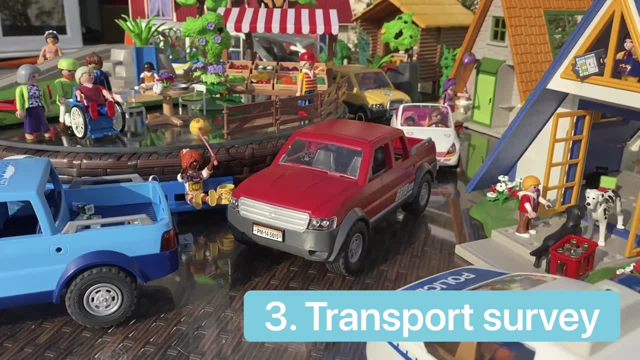 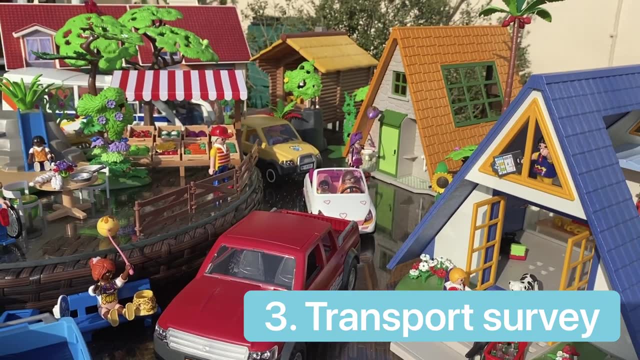 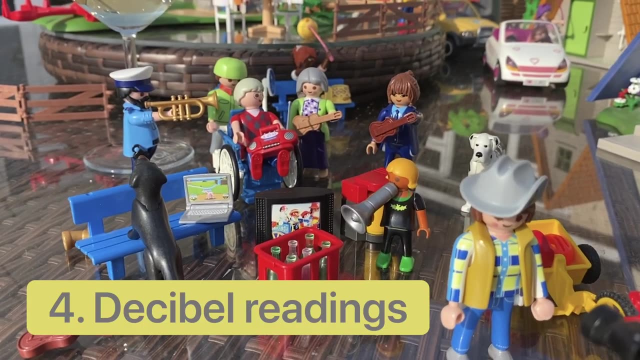 You can count the number and types of vehicles that pass your house. You could split these up into cars, lorries, vans. At the moment, you might see more delivery vehicles. Number four: decibel readings Using a free decibel app or the amazing Jogging. 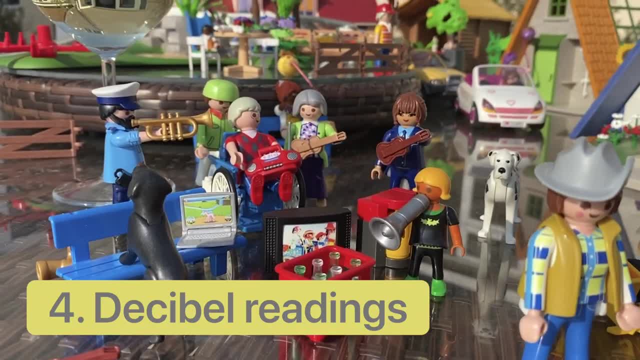 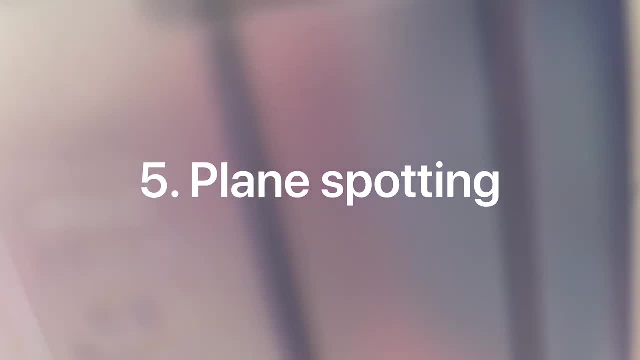 app you can record the exact most levels in your location. Number five plane spotting. Lie on your back and look up to the sky. How many planes can you see? Repeat this during the day, maybe every couple of hours? Are they less than? 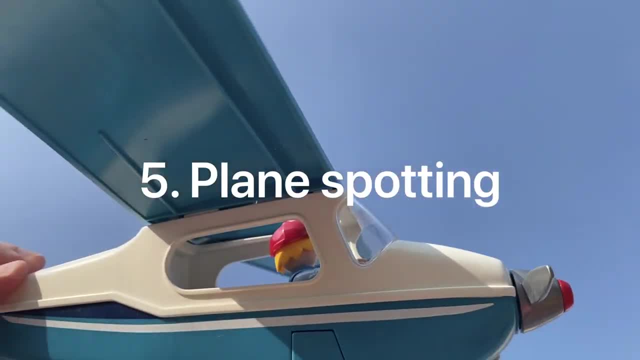 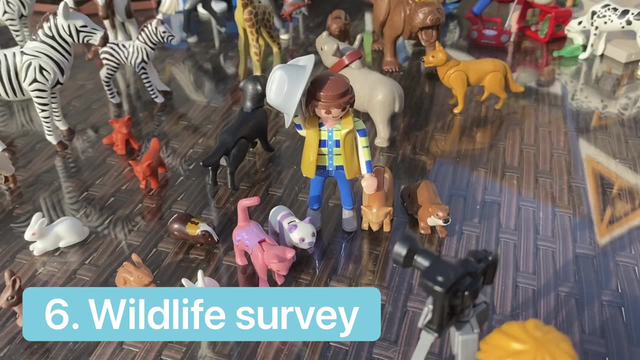 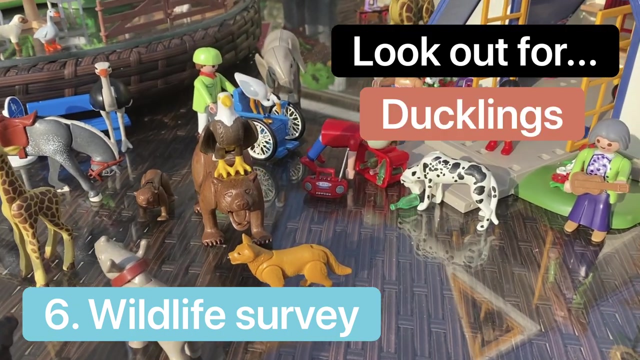 normal. Write down as many as you can. spot Number six: a wildlife survey. Keep a note that's by your window for a whole day and keep a note of all the different types of animals you can see from your house. You can. 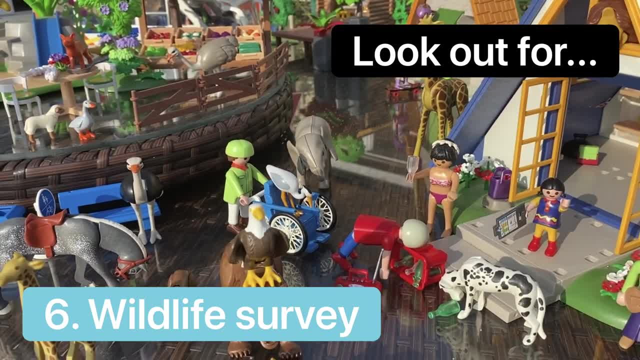 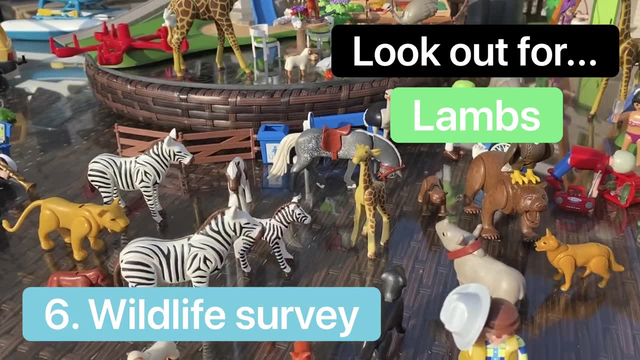 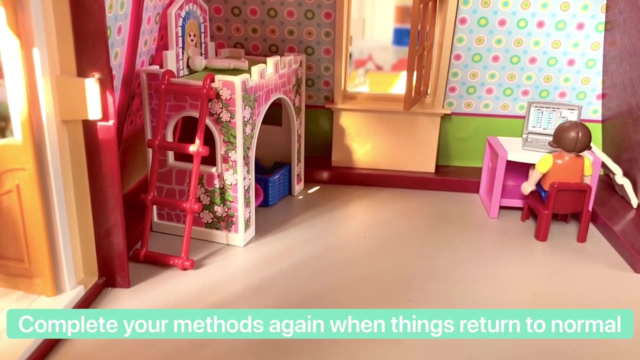 use a tally to keep a log of how many of each animal you can see and parts of the youth, such as fish, goats and deer, have been spotted in town centres. Once you have gathered your information, keep it safe. You'll be able to do the same thing. 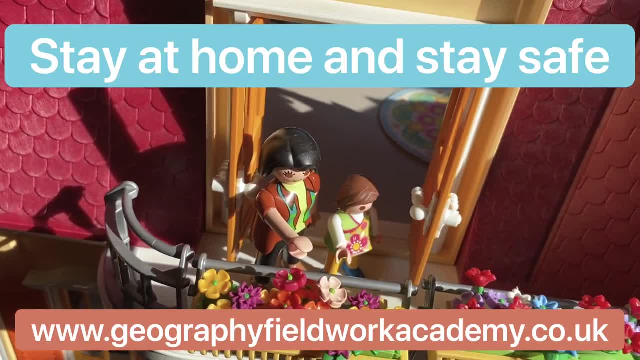 again when everything is back to normal. For more information, see our website. Good luck and stay safe. 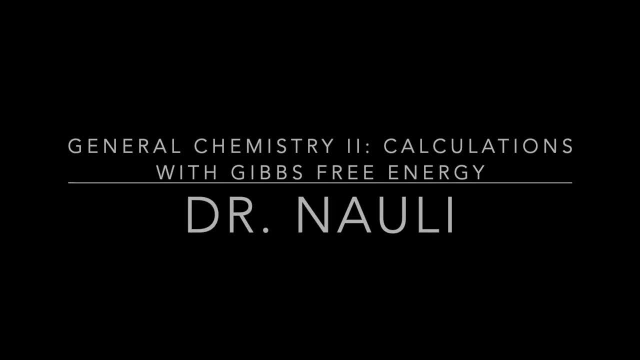 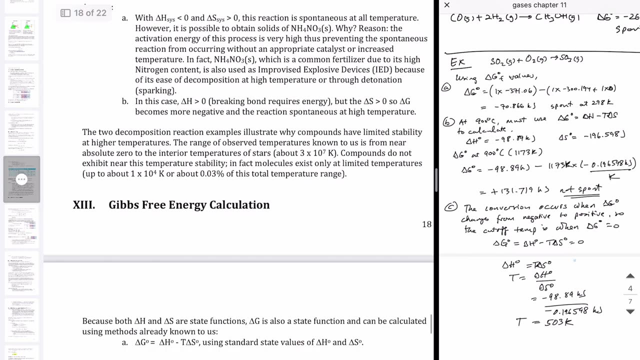 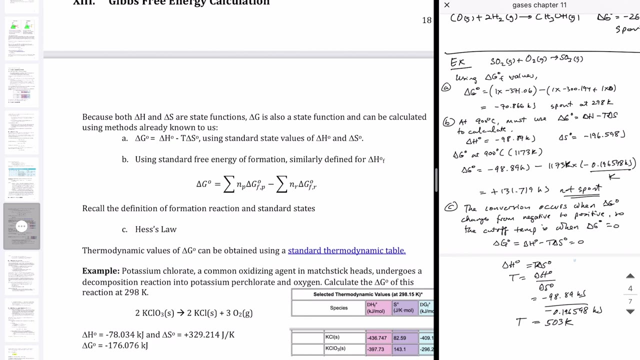 So we discussed how to determine the sign of delta G by looking at the enthalpy and entropy factors in the previous section. Now we want to actually calculate the value of delta and use that to determine whether our reaction is spontaneous or not. Again, keeping 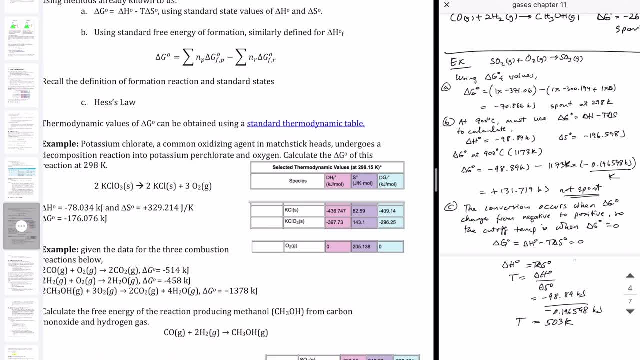 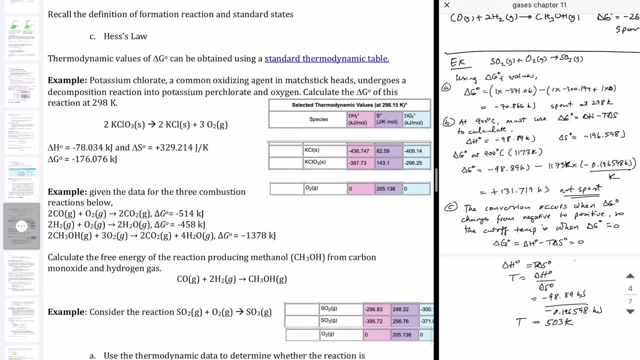 in mind that when delta G is negative, that's when reaction is spontaneous, and when it's positive it is not, and when it's equal to zero, we're at equilibrium for that given reaction. So let's take a look at these three examples Before we calculate them. I want 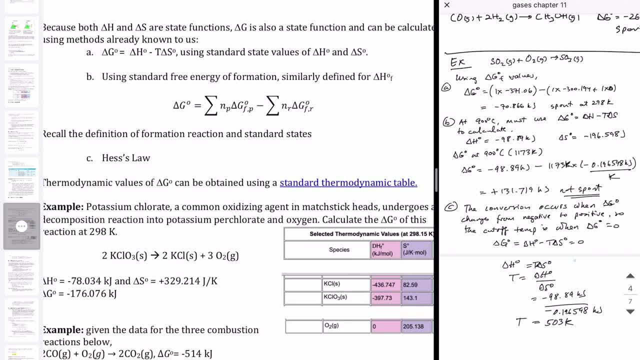 to remind you that there are three different ways to calculate delta G. The first one is just using that delta G equal to delta H minus T, delta S equation that we looked at in the previous section. The second one is very similar to how we calculate the change. 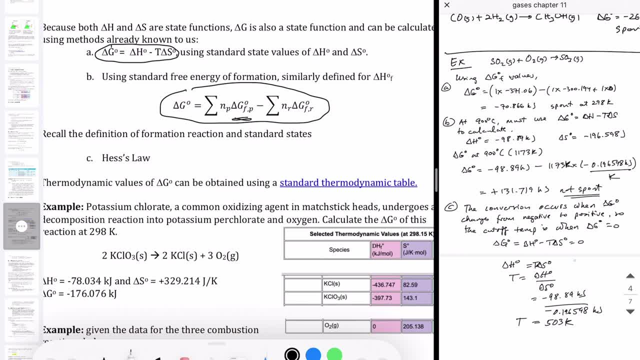 in enthalpy, delta H, which is using these enthalpy of formation values. Here we're going to use something called the Gibbs- free energy of formation- to help us calculate the value of delta G, and the formula is the same. You take the product's. 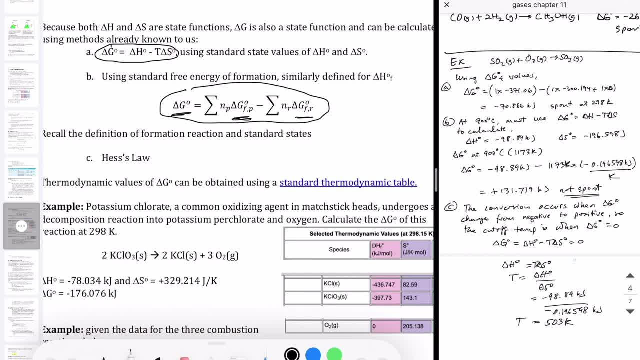 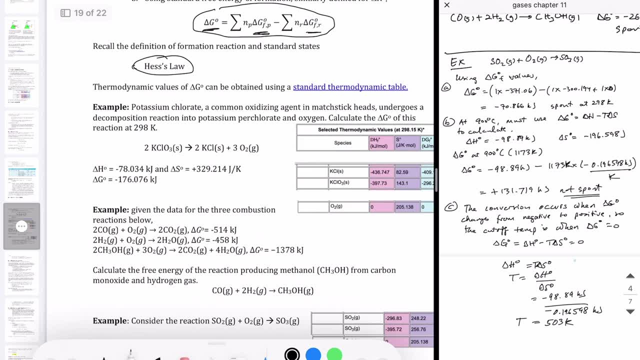 value minus the reactant value, with each of the species multiplied by their stoichiometric coefficient. And then the last way to calculate delta G is Tesla's law, which is the same concept we use to calculate delta H. Let's look at these examples now. The first one: